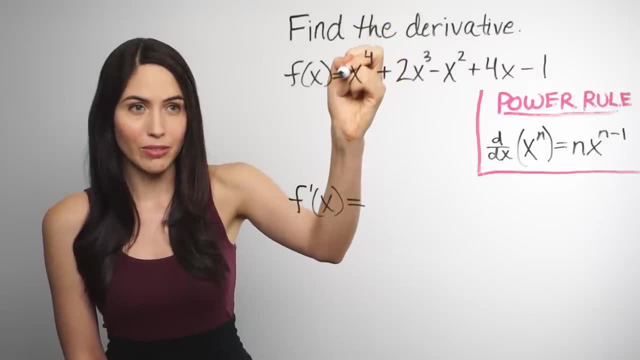 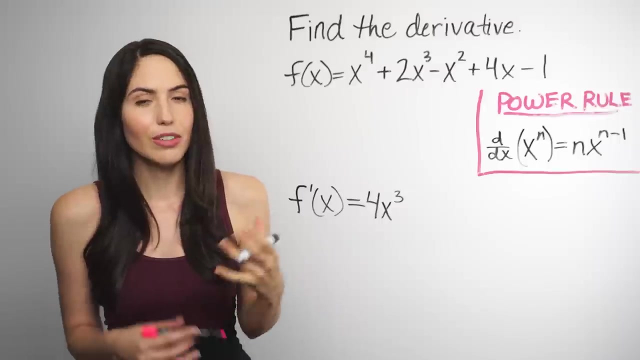 So for this one we bring down the four to the front as a coefficient and then reduce that power by one. So instead of x to the fourth we're going to have x to the third, And that's it. That's all you have to do for that term. 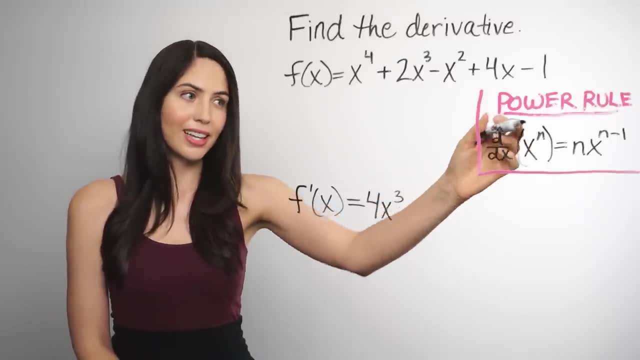 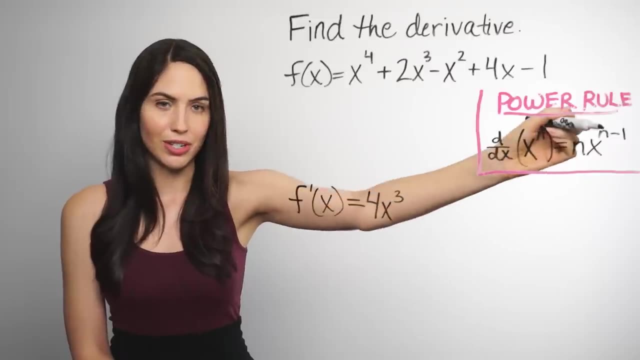 And technically this is the power rule. if you want to see it to take the derivative of x, You have a power of x. You bring down the power out front as a coefficient and then reduce the power by one. This is for positive integer powers. 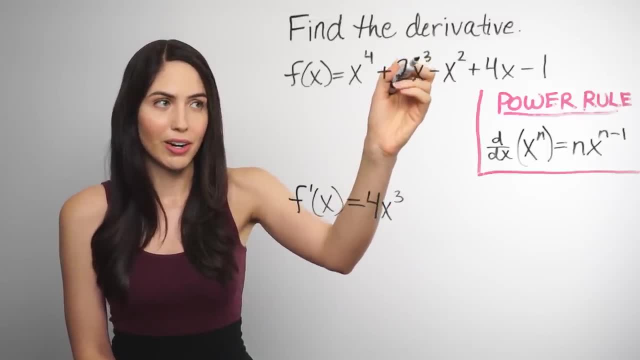 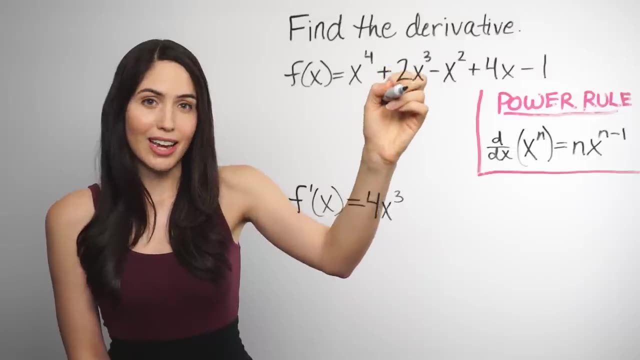 So let's look at the next term, 2x to the third power. This looks very similar, but it has this 2 multiplied in the front. When you have a constant multiplied in the front of the term, you can keep the constant and then take the derivative of the rest of the term. 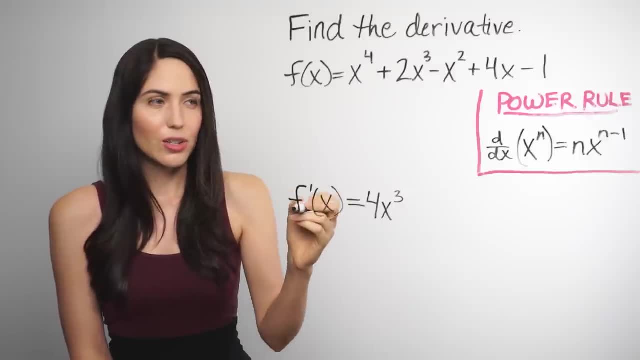 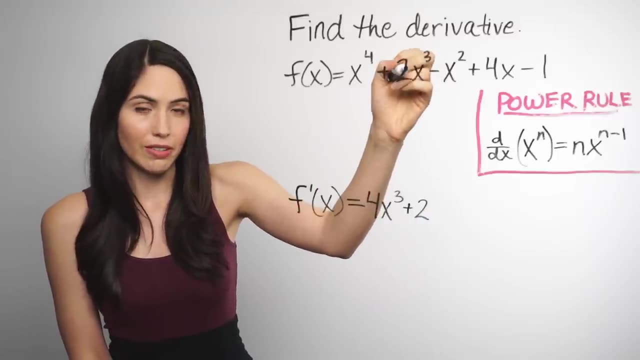 That's the constant multiple rule, if you see that. So we keep the 2, and then we take the derivative of the rest. so we take the derivative of x cubed using the power rule, since it's the power of x. 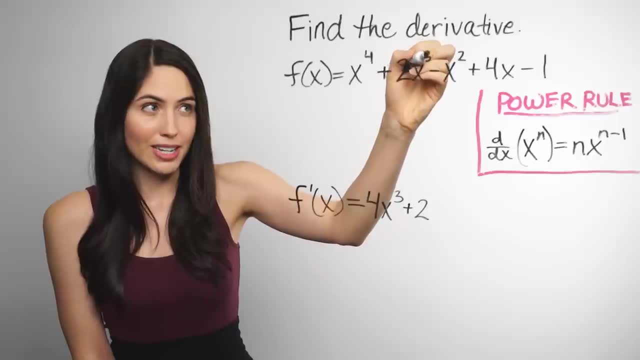 To do that, we bring down the power of 3 to the front as another constant multiplied, So times a 3. And then reduce the old power 3, by one. So instead of x cubed we have x squared. 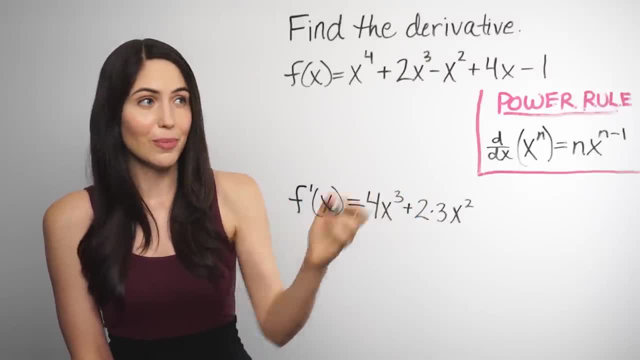 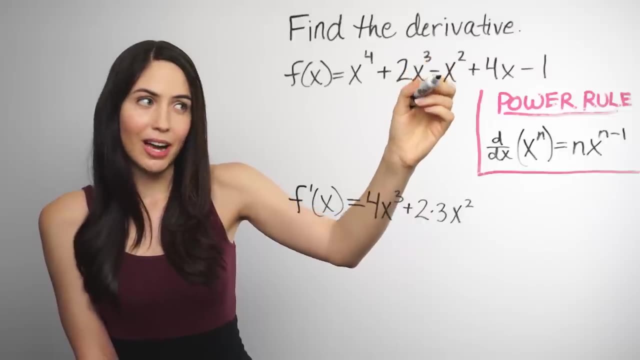 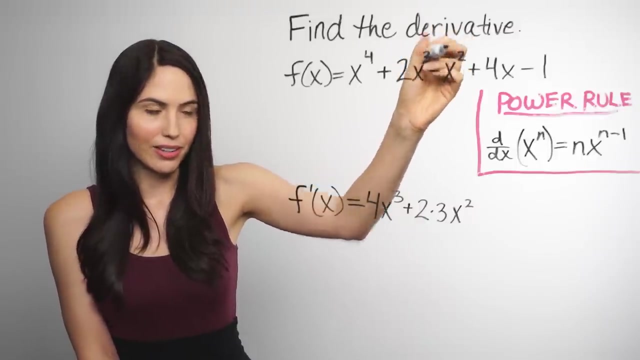 Great Next term minus x squared. So we're subtracting x squared. How do you find the derivative of x squared? It is a power, so power rule. Again same story. You bring down the 2 out front and then reduce the power. 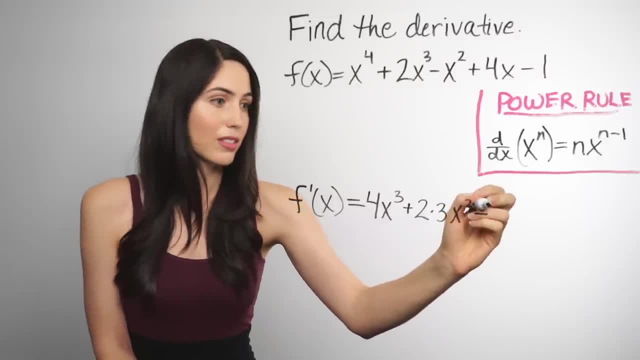 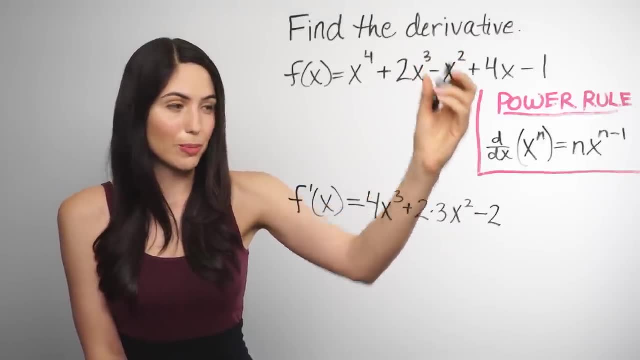 And it's still subtraction. Bring down the 2 out front, reduce this power. so instead of x squared, we have x to the first power. You don't have to write the 1 power, but I'm going to write it for now. 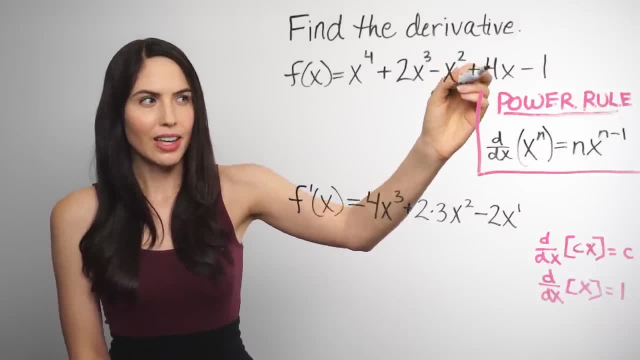 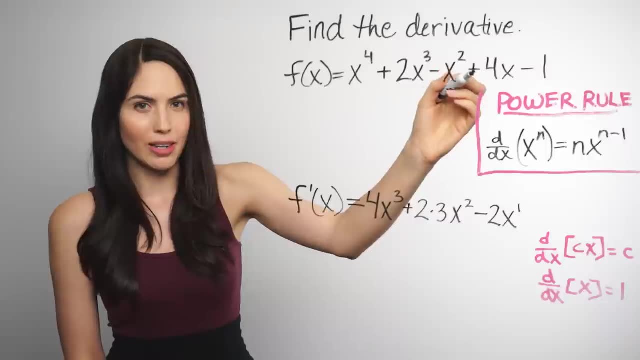 Okay. so look at this next term plus 4x. Anytime you have a number times x, 4x, 2x, 10x, the derivative of that term will just be the number. So the derivative of this will just be 4.. 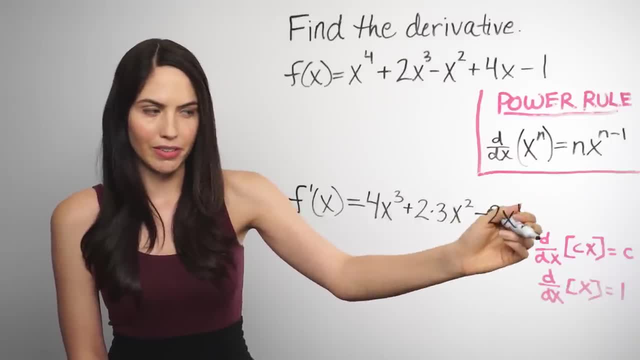 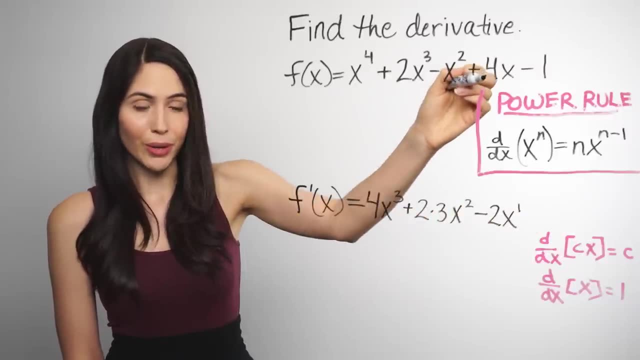 You can think of this as a separate rule, some people do. The derivative of a number times x is just that number, Or some people think of it as the constant multiple rule. You have this 4 in front, so you keep the 4,. 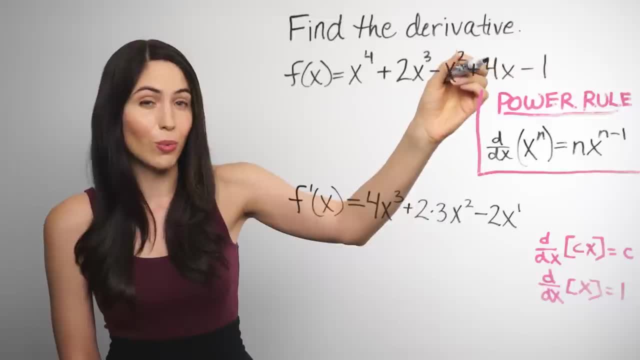 and then take the derivative of x. The derivative of x is 1.. Why is the derivative of x 1?? Because of the power rule, Because x is technically x to the first power, x to the 1.. And if you use the power rule on x to the 1,, 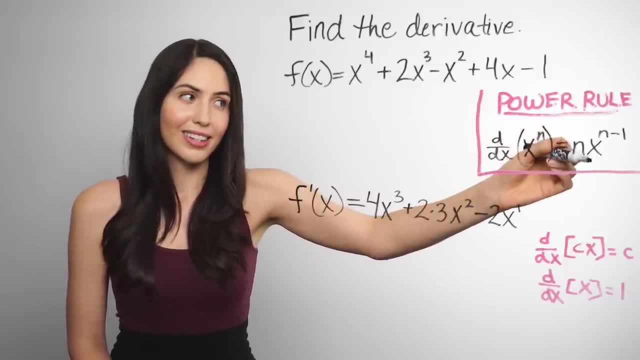 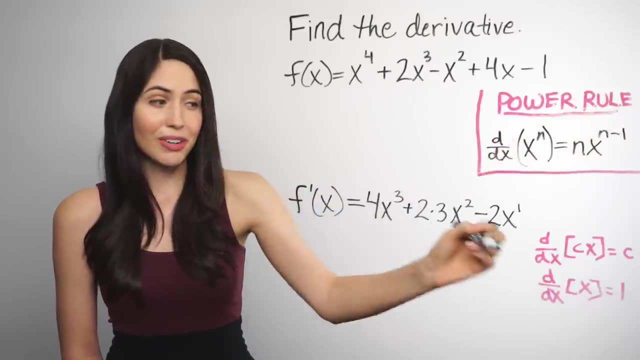 you get 1x to the 0, because you're reducing the power. x to the 0 is 1, so you have 1 times 1,, it's 1.. The derivative of x is 1, and you can just remember that if you want. 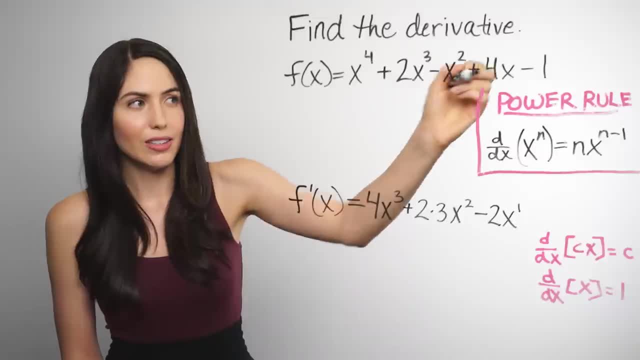 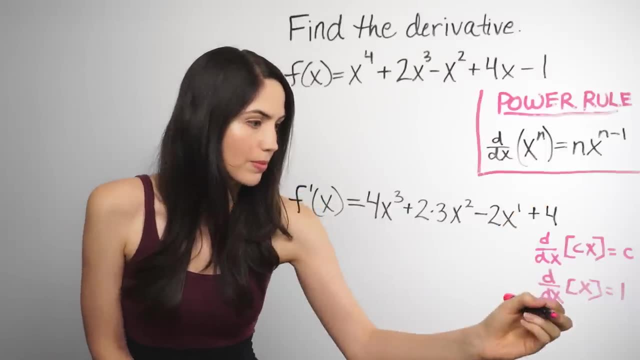 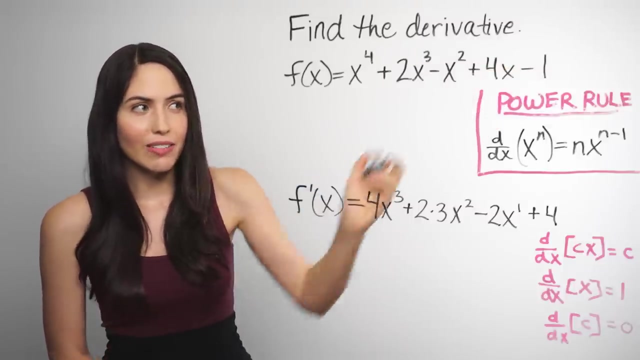 Most people do. But any way you look at it, the derivative of this term is 4.. Okay, last term, this minus 1.. This is great, because anytime you have a number or a constant by itself, the derivative will just be 0.. 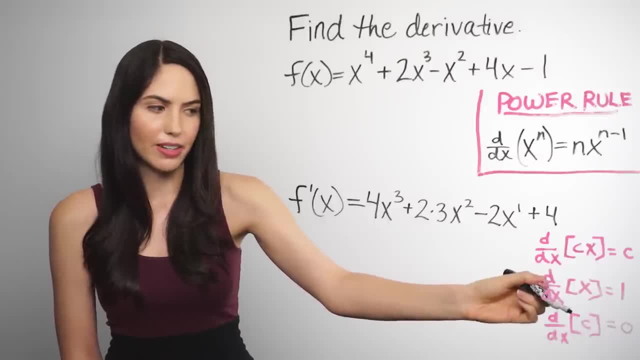 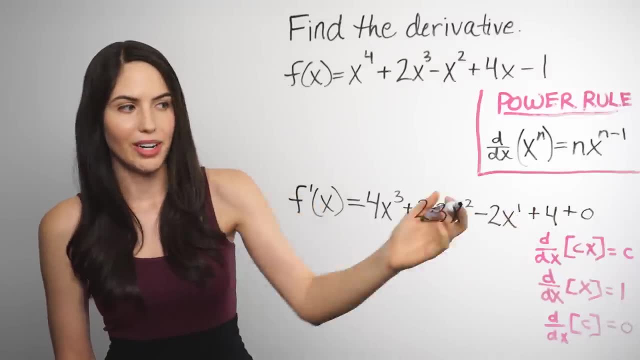 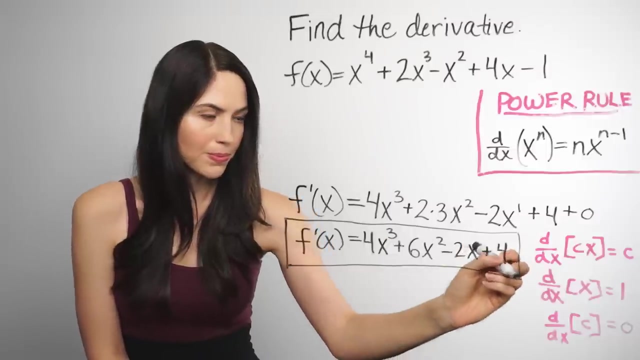 It's nothing. That's actually a rule: the constant rule. The derivative of a number constant is 0.. So for now, we can write plus 0.. Let's just clean this up a little bit, Alright? so this is the answer. 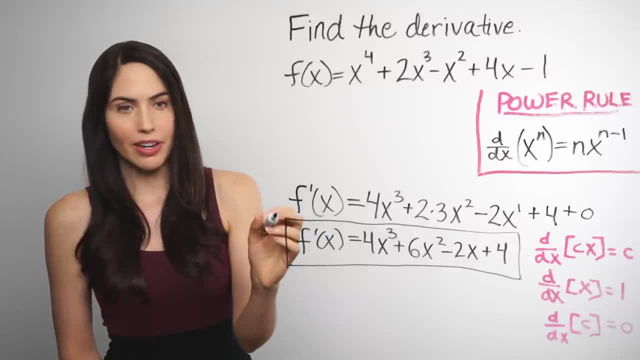 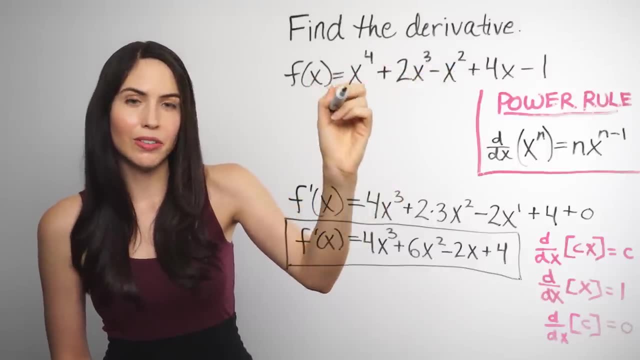 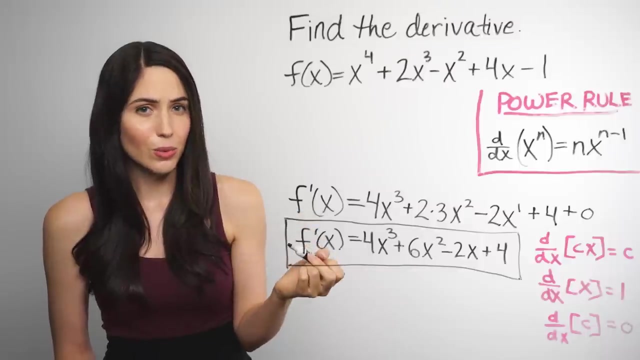 This is the derivative And we were able to find the derivative by differentiating each term individually. All these terms that were added or subtracted, we could take the derivative of each of them individually and string them together for the full derivative. That is the sum and difference rule. 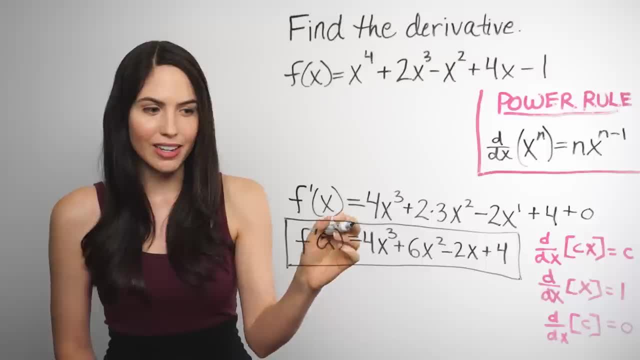 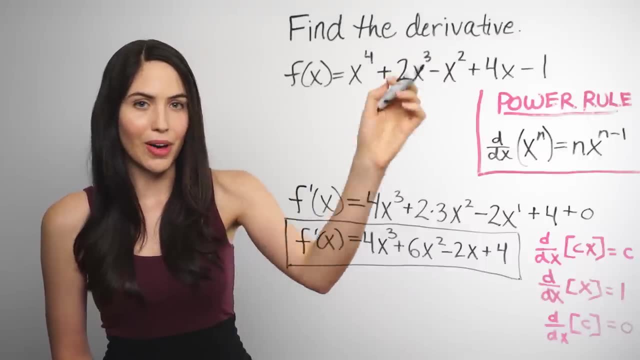 You see that. More rules to remember, But that's what that is. And f, prime of x, the derivative, tells you the rate at every x value of that original function. f tells you the slope or instantaneous rate of change: Slope of the tangent line or instantaneous rate of change. 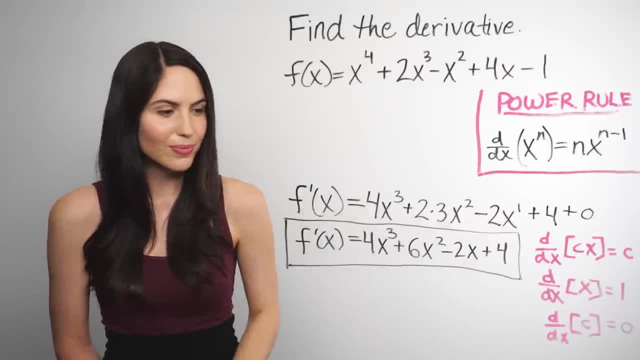 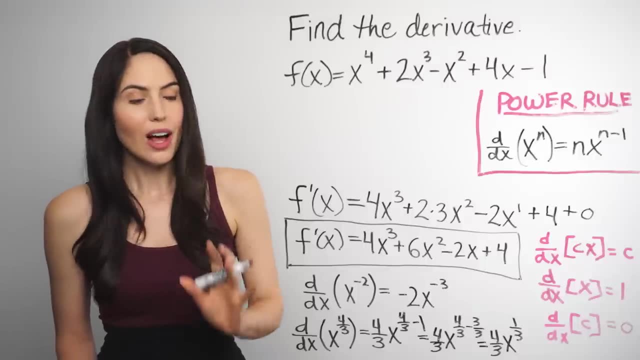 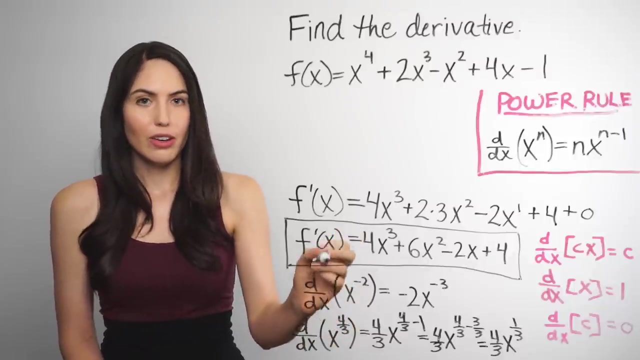 of the original function. Okay, so, by the way, it's the same idea. if you have a negative power or a fraction power or a rational power For a negative power, as long as x is not equal to 0,, you can do the same thing. 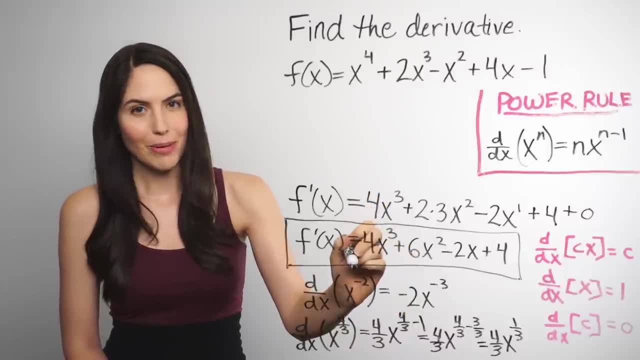 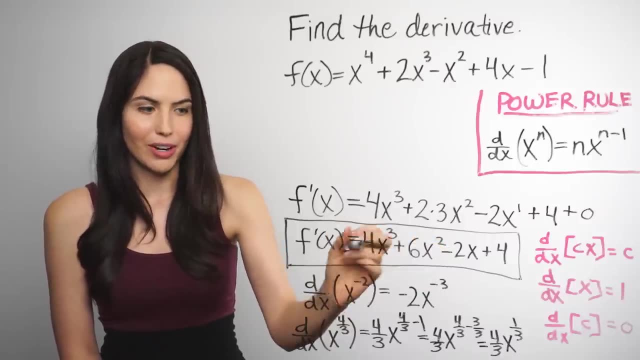 Bring down that power to the front and then decrease the power by 1.. But watch out for negative powers. Reducing that by 1 means you get a larger negative number, a more negative number. So negative 2 minus 1 is negative 3.. 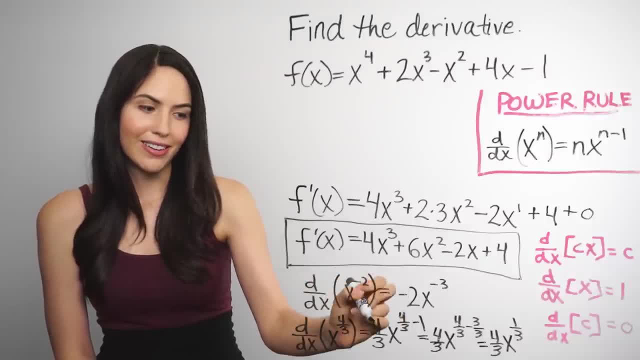 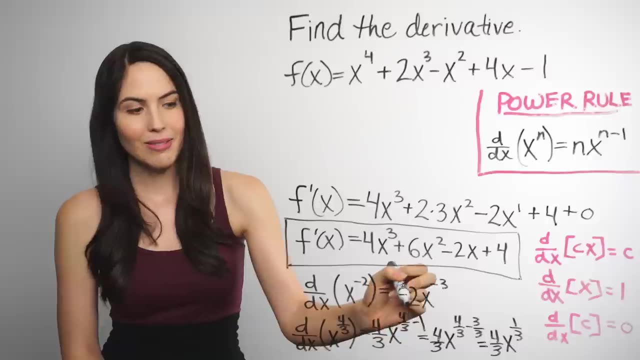 And then for a fraction power, same idea. You can bring that down as a coefficient up front. Subtract that original power by 1. And because you have a fraction minus 1, an integer, you'll need to get a common denominator to find the new power. 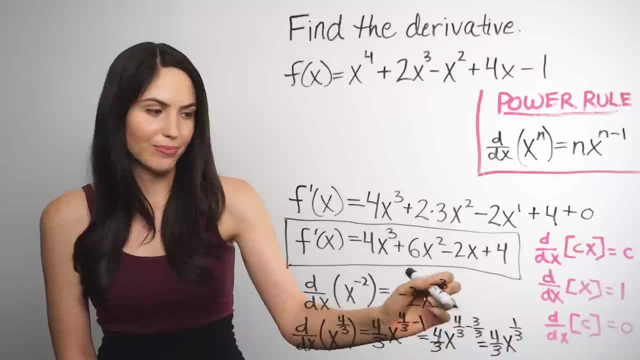 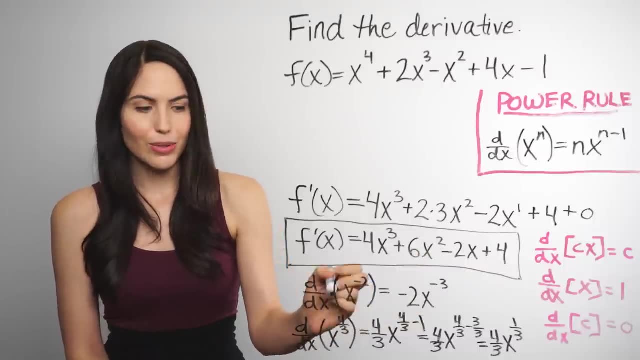 And that's probably a throwback to middle school- Getting a common denominator come back to haunt you. But if you do that, you'll get the right power for the answer. The only thing with this kind is if you start with a fraction power. 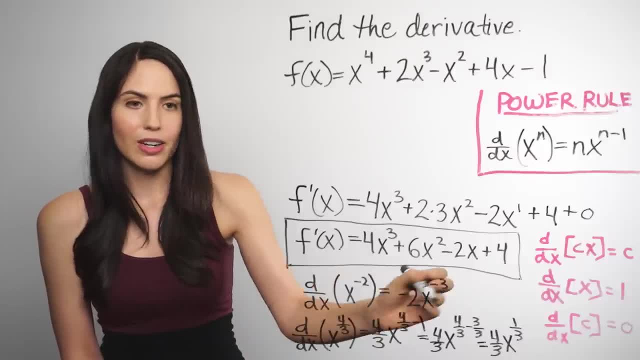 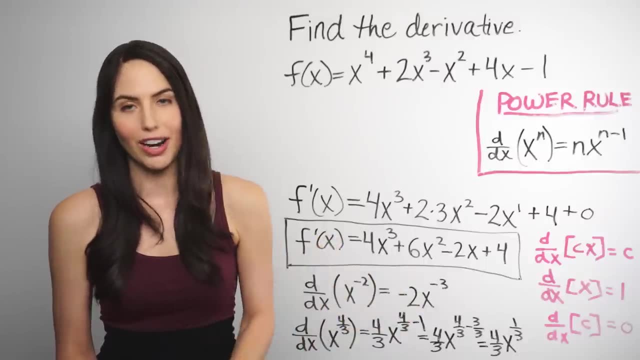 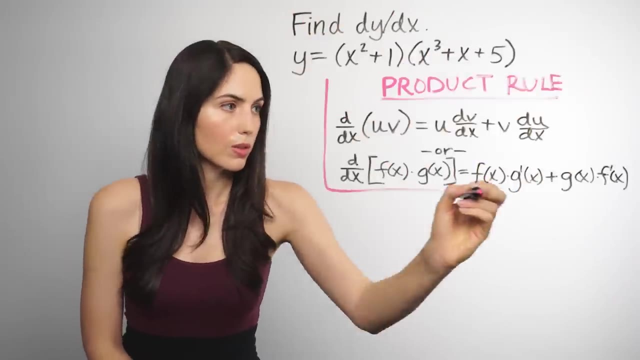 that's less than 1, like 1 third. the derivative that you end up with won't be defined at x equals 0. But in general it's the same idea for negative powers and fractional powers. Okay, so say your equation. 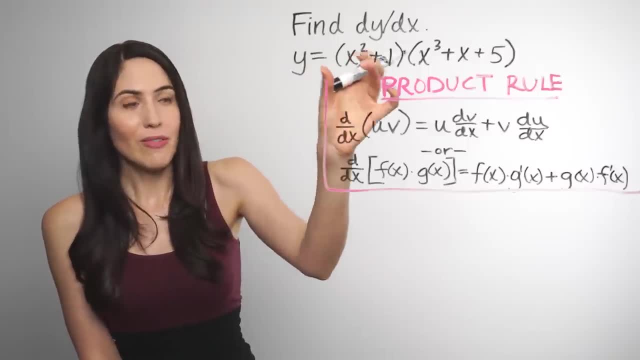 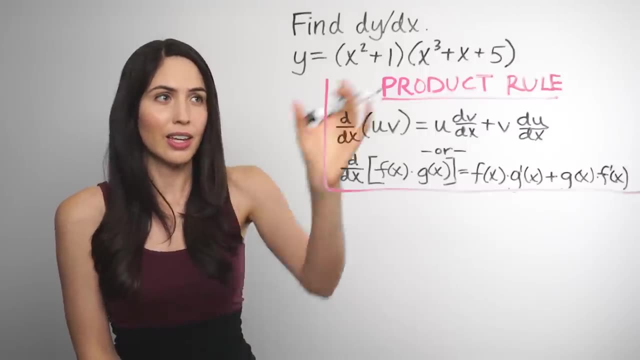 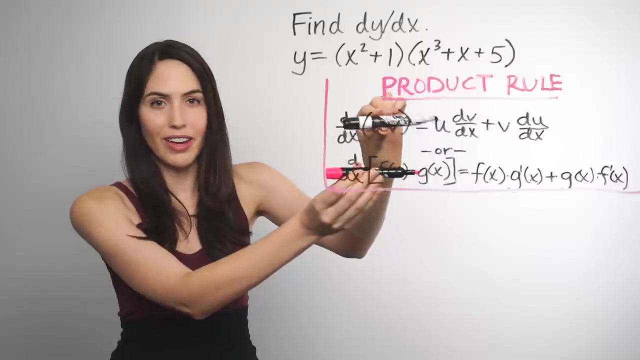 is not just a polynomial, but is one factor multiplied by another. If your equation has the overall form of one thing multiplied by another, you're going to want to use the product rule. Here's the product rule. I've given you two forms of it. 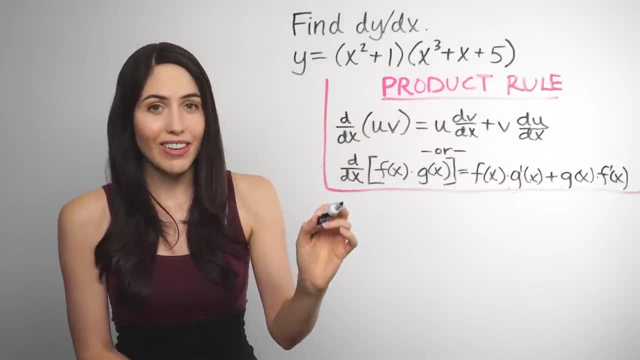 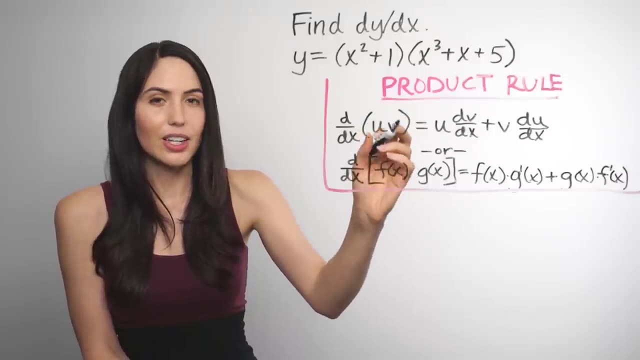 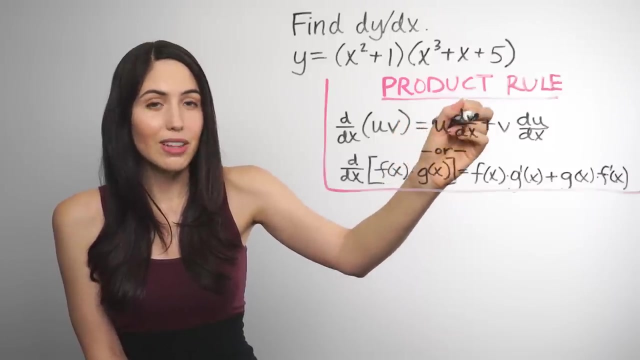 They mean the same thing, It's just different notation. But the gist of it is that to take the derivative of two functions multiplied together, u times v, you just have the first function, as is times the derivative of the second function, plus the second function, as is. 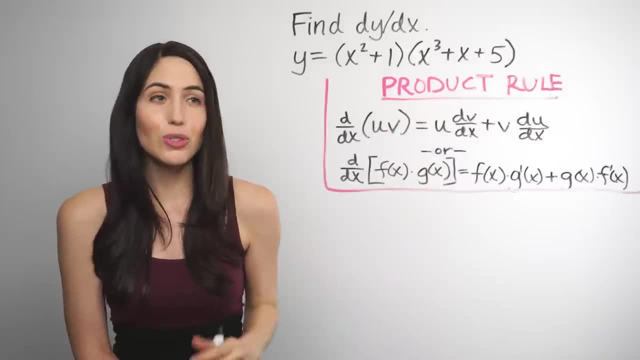 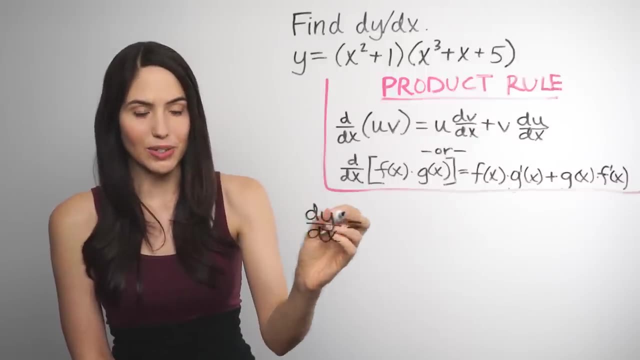 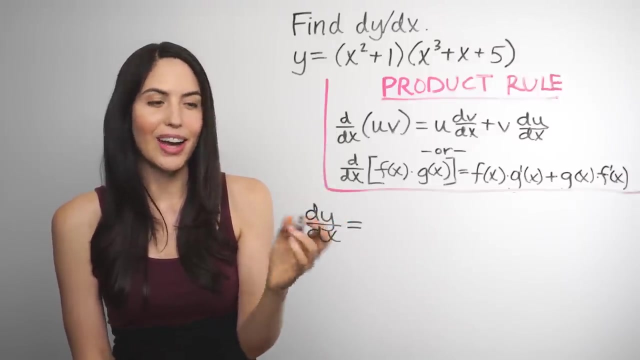 times the derivative of the first function. So that's it. So let's try it for our equation. So dy dx equals. This just means the derivative of y dy dx. This is different notation from before. I know I gave you Leibniz notation this time. 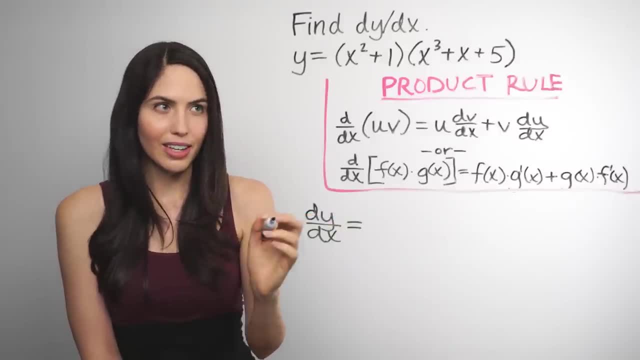 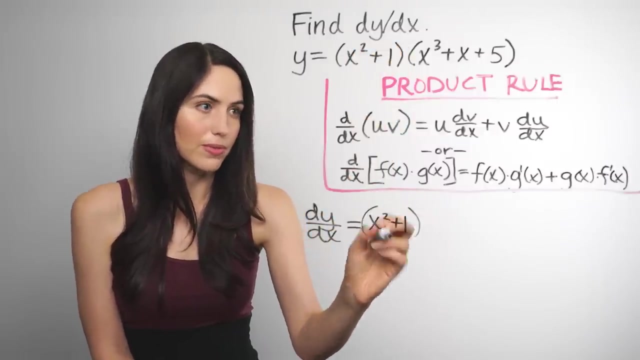 for those of you who feel strongly about notation, We'll use the product rule. The product rule says: first write the first factor as is first factor, as is x squared plus 1, times the derivative of the second factor, times the derivative of this. 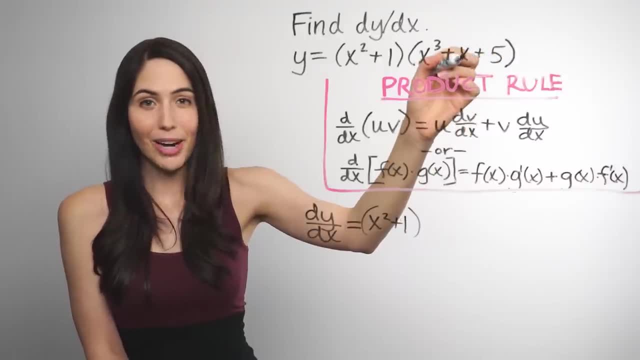 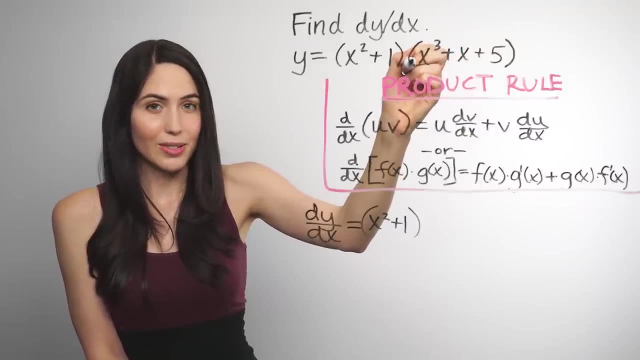 x cubed plus x plus 5.. Oh look, it's the power rule. We can take the derivative of this term, x cubed. with the power rule We get 3x squared. Derivative of just x is 1,. 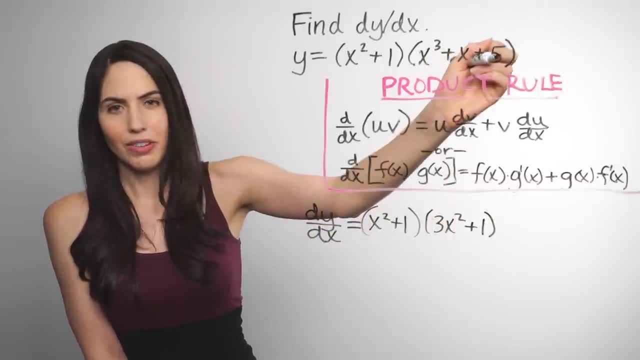 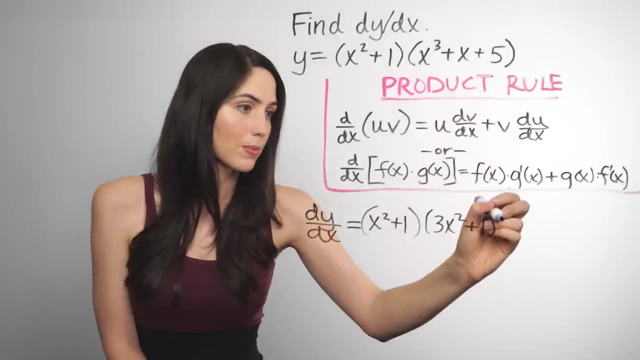 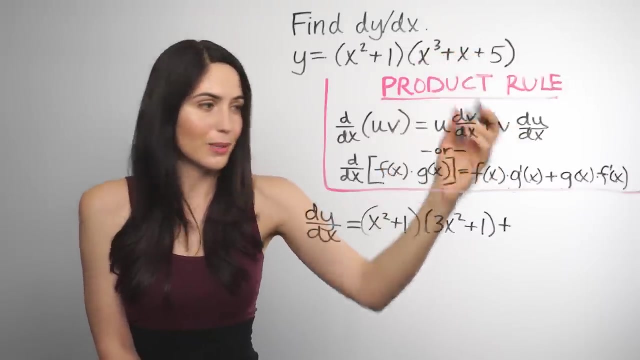 so you have plus 1.. And the derivative of 5 is nothing, so that contributes nothing And we're not done. We have plus the second factor, as is this, as it is finally- times the derivative of the first factor. 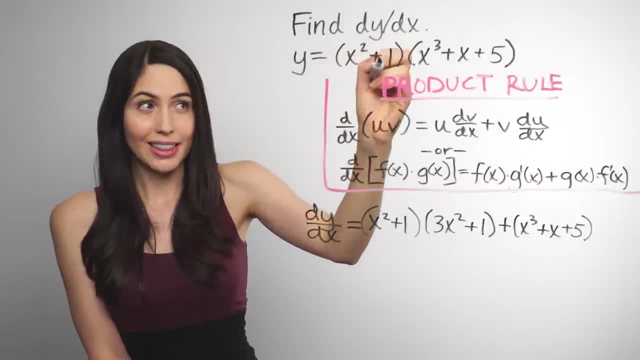 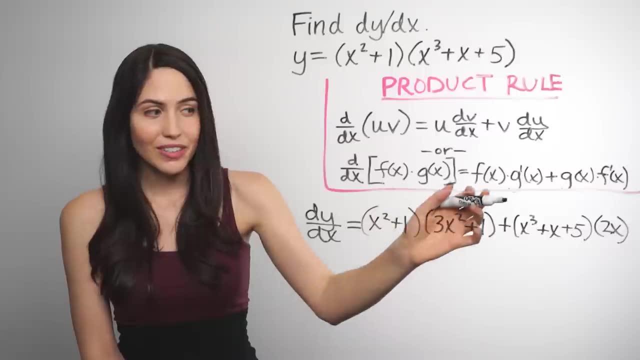 The derivative of just this is 2x and then nothing from that. So just 2x for all of that, And that's it. That's the derivative, That's the answer, If you want to or if you have to. 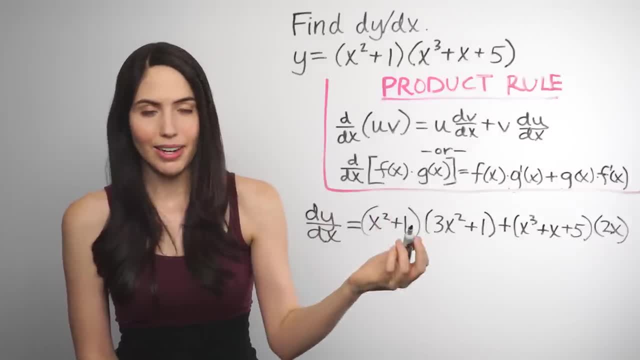 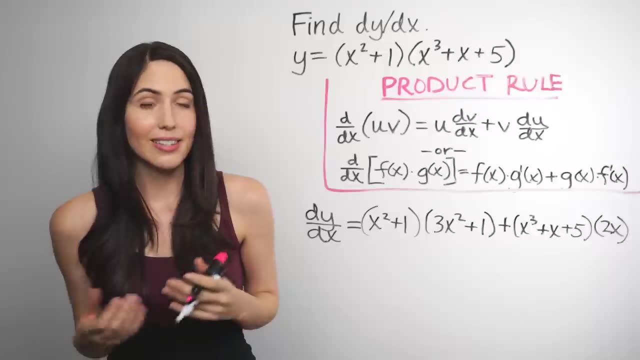 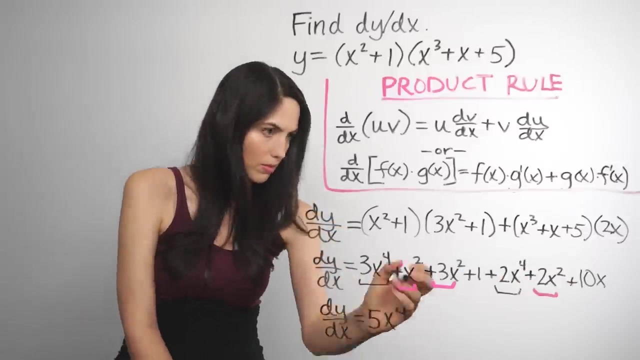 you can simplify this. Multiply it out, combine like terms and simplify. You probably should do that because reasons It's neater, You'll get a simpler result. So let's do it, Okay, so that's the answer. 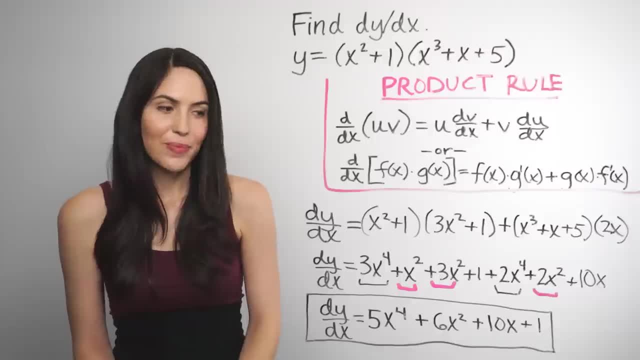 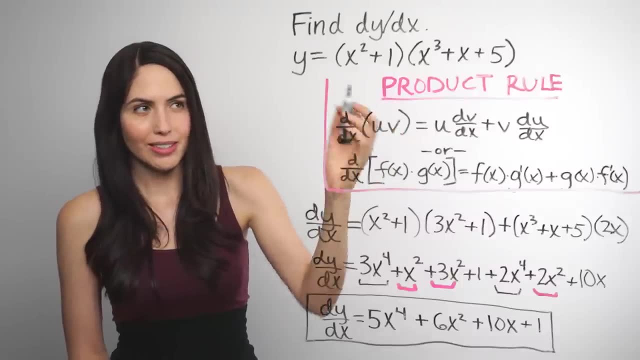 the simplified answer for the derivative. That's all we have to do. And for this particular one, just so you know, you could have done it without the product rule. in this case, You could have multiplied this out, distributed this all out. 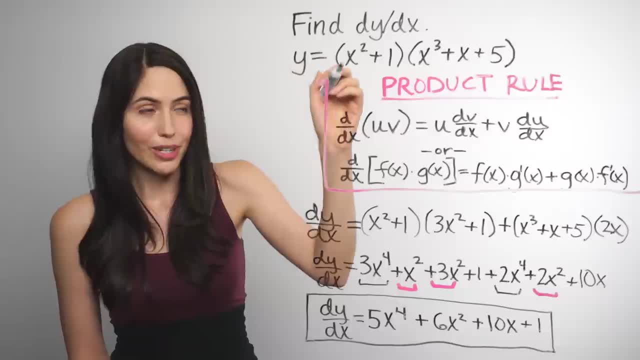 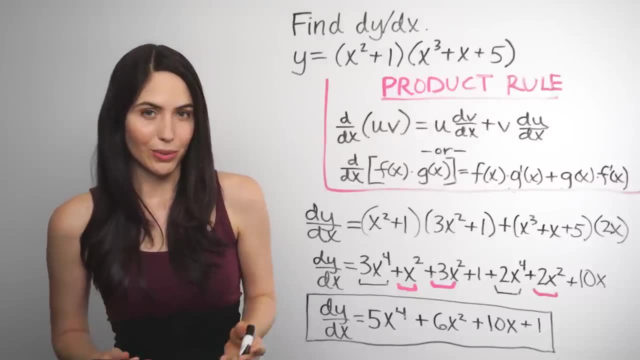 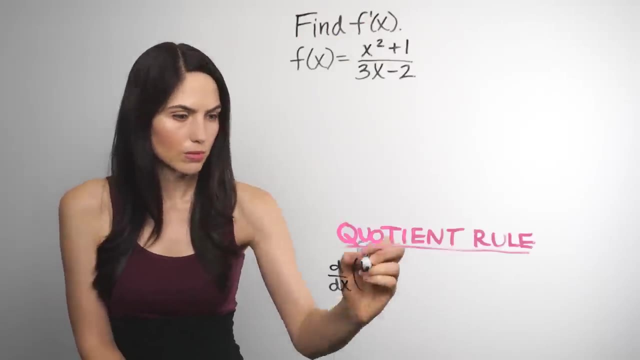 foiled it and then used the power rule on each separate term. You could do that whatever if you prefer that, But at some point you're going to want the product rule And this is how you use it. Okay, so if your equation 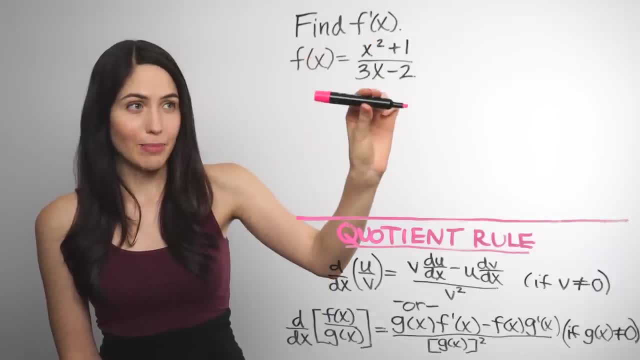 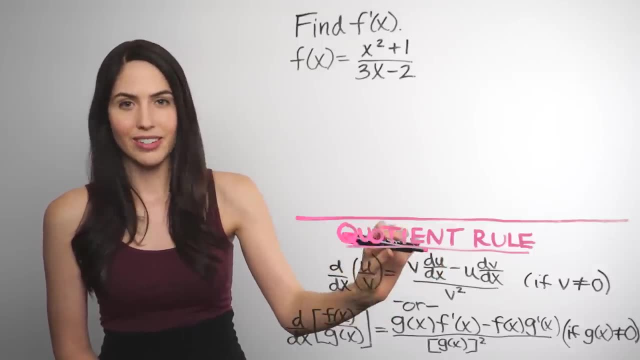 has the overall form of one thing divided by another and you have to find the derivative. you should use the quotient rule And I've given you two forms here. They're just different notations. They mean the same thing. I know this looks a little. 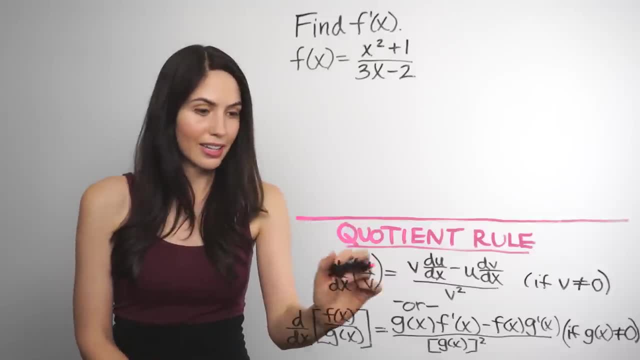 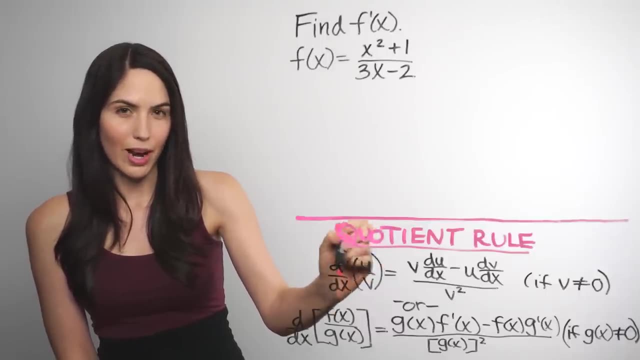 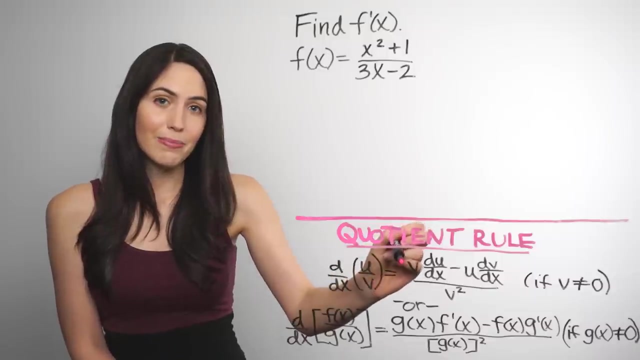 barbaric and medieval. Don't worry, All it means is that if you have one thing divided by another, we'll say a top and a bottom in your rational expression. to take the derivative of that quotient, it's just the bottom times the derivative of the top. 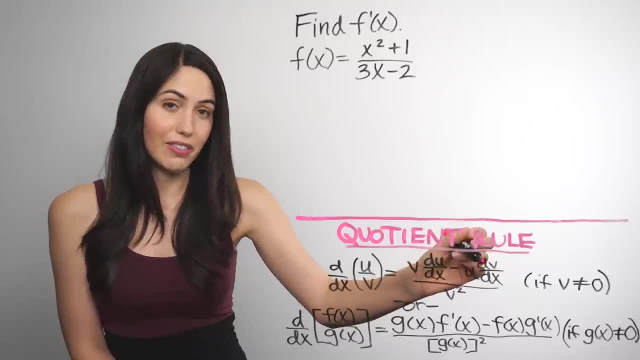 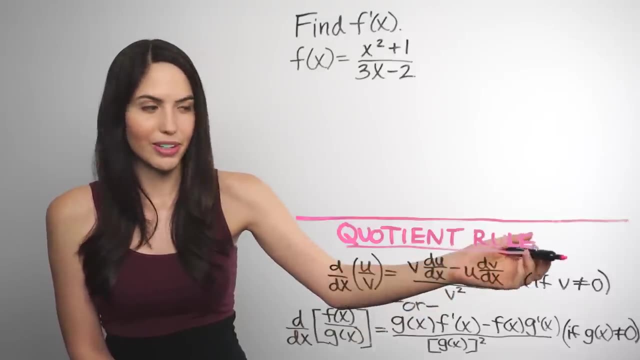 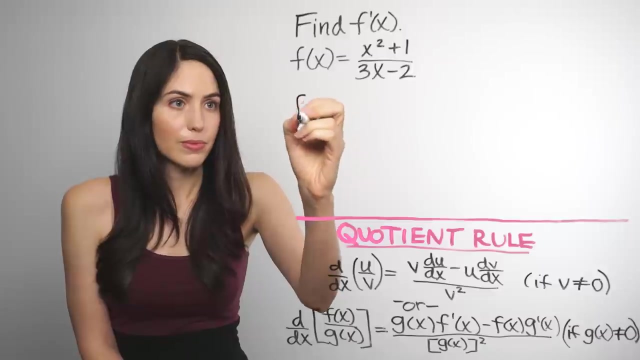 minus the top times the derivative of the bottom. all over the bottom squared, The bottom times itself As long as the bottom is not equal to zero. But that's all you do, So let's try it for this function. The derivative f, prime of x. 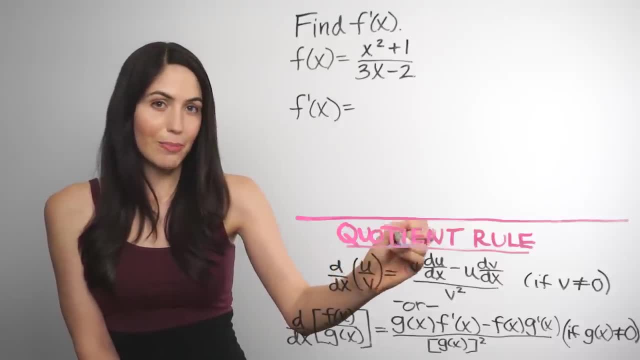 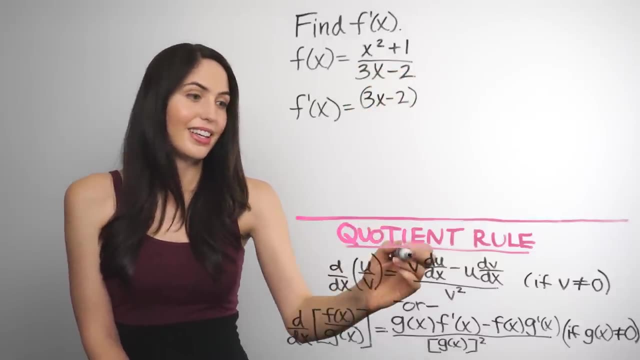 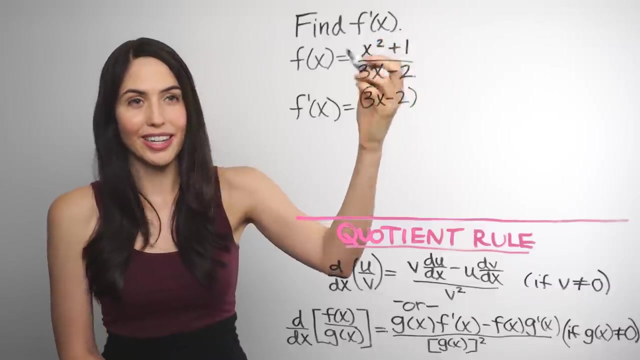 First, with the quotient rule, we write the bottom, as is So 3x minus 2.. Then times the derivative of the top, the numerator, The derivative of x squared plus 1.. Hopefully you're getting the hang of this. 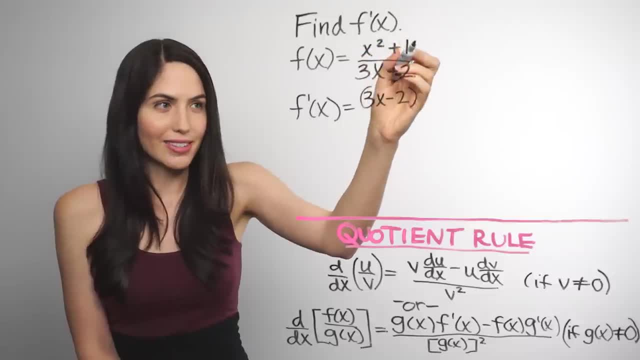 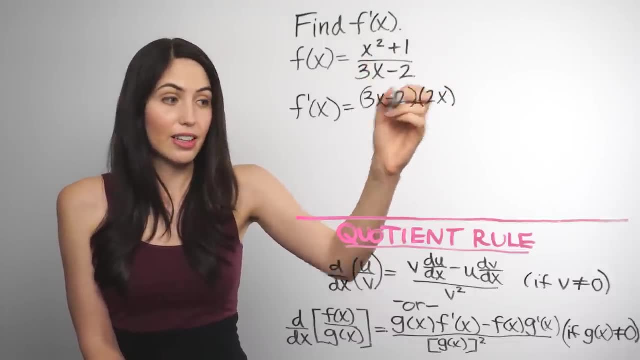 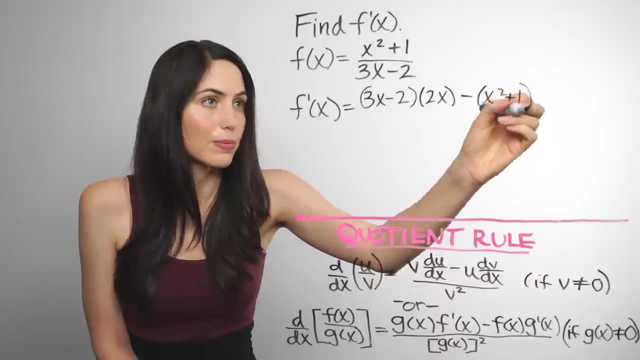 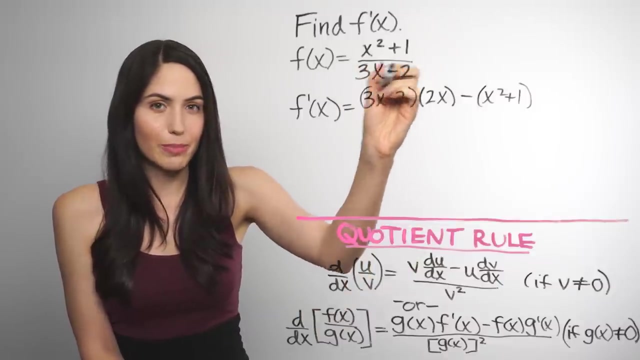 Would be 2x plus nothing. So 2x, It's just a straight up power rule. Then we subtract, minus the top as is, So just the top part, as it's written Times, the derivative of the bottom, The derivative of 3x minus 2. 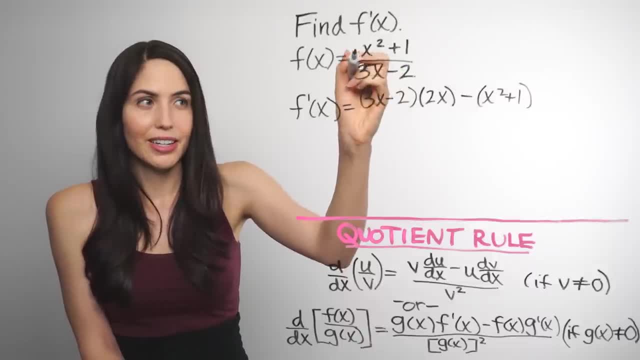 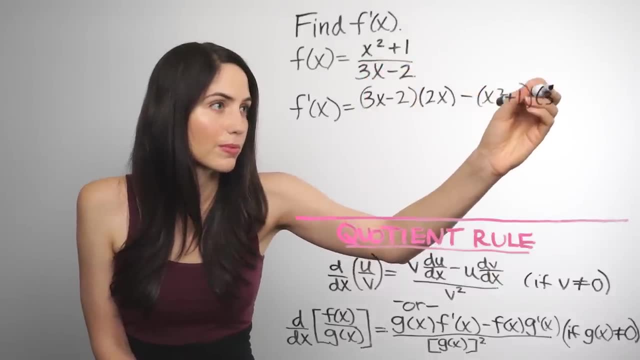 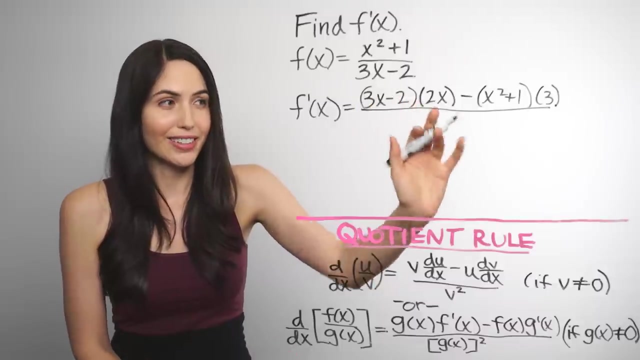 will just be 3.. Because this term gives you a derivative of 3.. And if you differentiate, a constant, it's nothing, It's zero, It's a 3.. Then it's all over divided by. humor me, we're almost done. 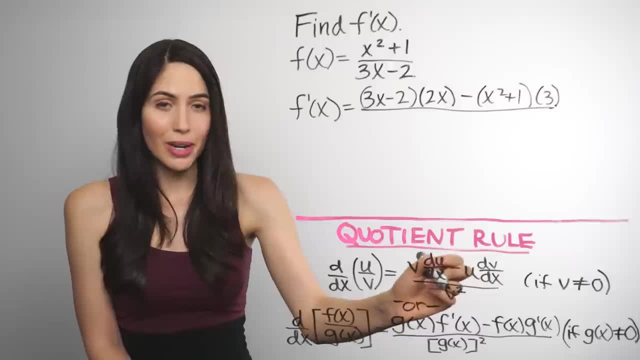 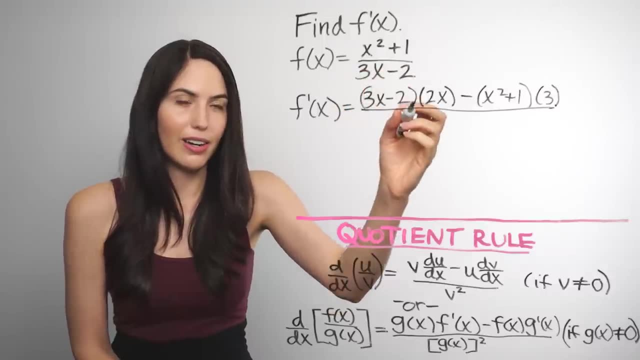 There is a method to this madness. I promise: Just the bottom part squared, So just the denominator times itself, So we can write that as 3x minus 2, all squared in the denominator. So that's it. That's the derivative.